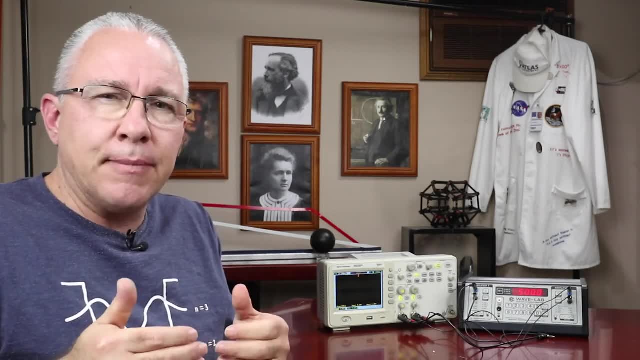 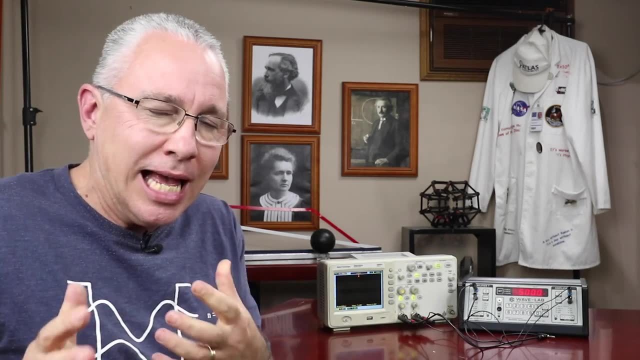 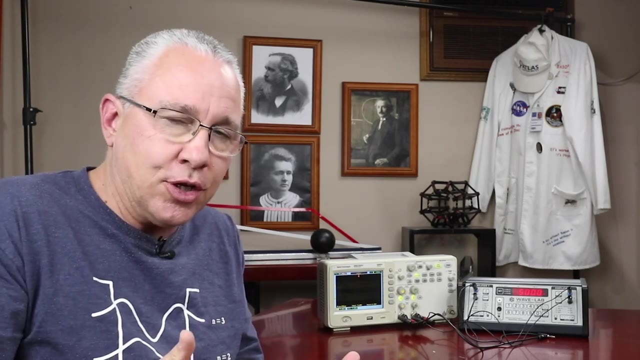 the signal from my phone onto the light, that information was able to be processed to therefore get some sort of sound out of my speakers. In essence, what's happening is that the information is somehow impressed on a carrier wave. Now, in the example I showed you just a second ago, the 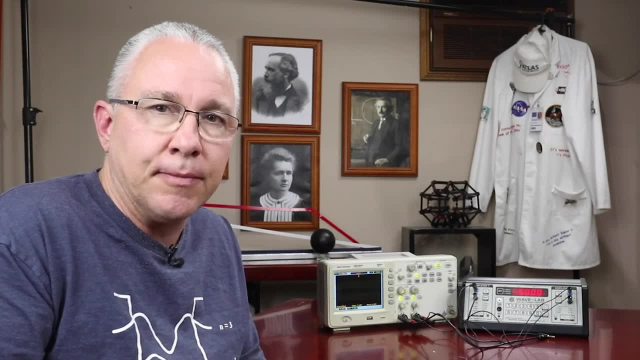 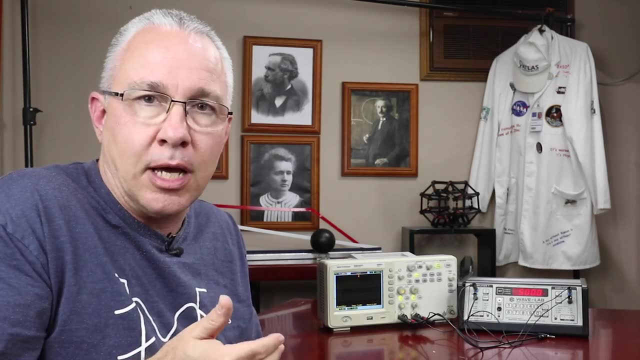 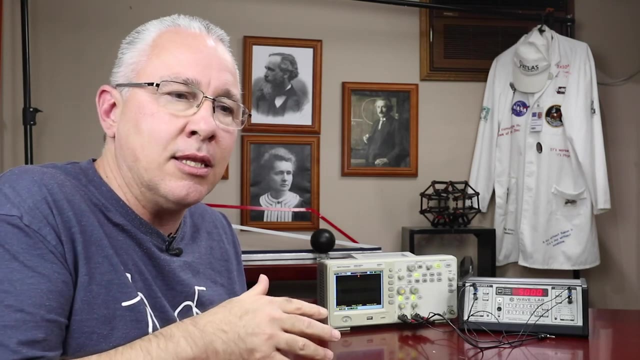 carrier wave was light or the visible light part of the spectrum, And in some way I was able to put information onto that visible light spectrum or those visible light frequencies, And what was able to be occurring was I was able to transfer that information on and then the small box was. 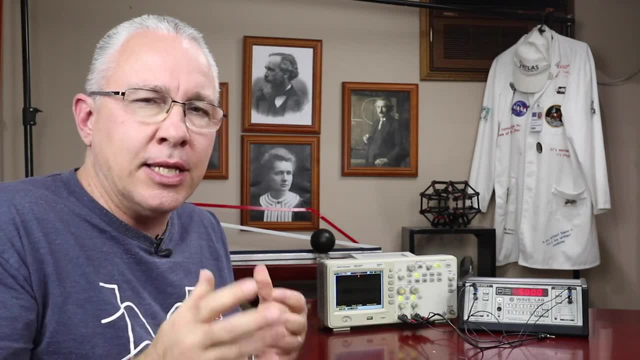 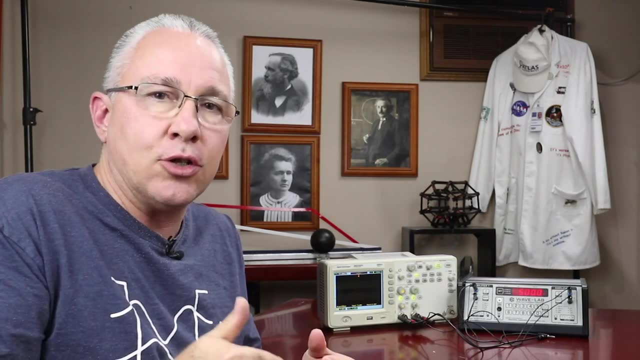 able to remove that information off. So really there's two number of processes going on here And in essence what this is is called is modulation. So adding that information onto the carrier wave is called modulation, And then removing or extracting that information to be 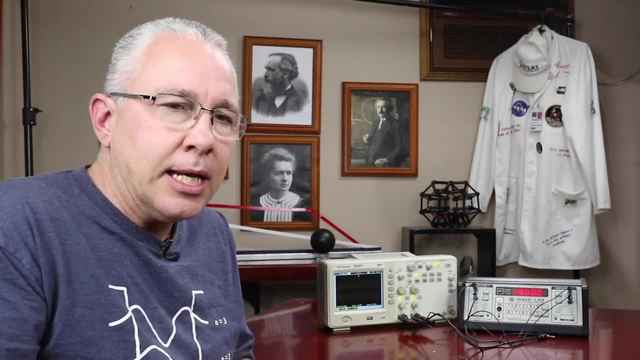 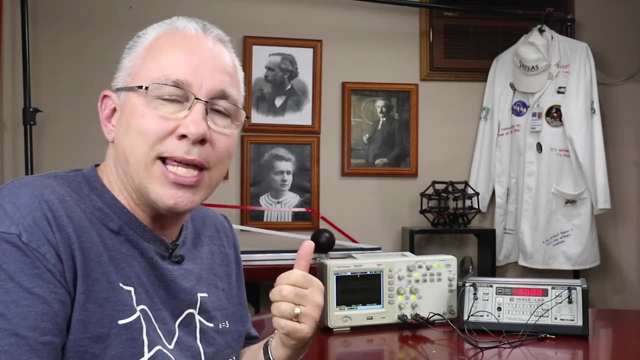 therefore transmitted to the speakers, is called demodulation. Now, today I'm going to be discussing only the analog versions of modulation, That is, in specific, we're going to deal with amplitude modulation and frequency modulation, And there's also phase modulation, which I'm not 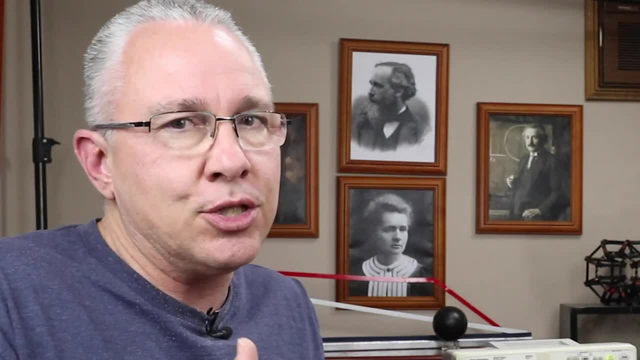 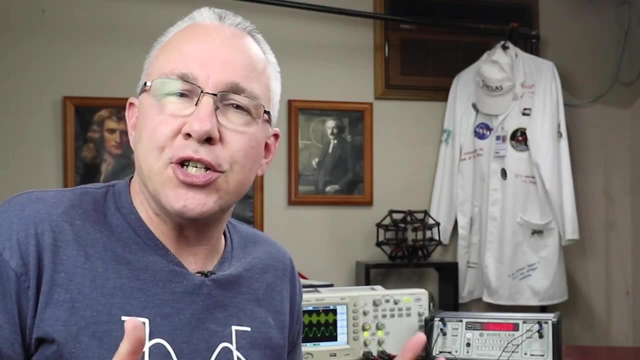 going to discuss. And then there's also digital modulation, which is a whole section again and not part of this video. This is really about the basics of modulation. So what does modulation actually look like? So what I have here is an oscilloscope that's receiving 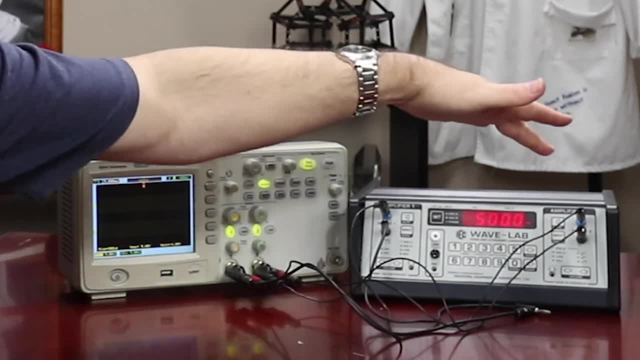 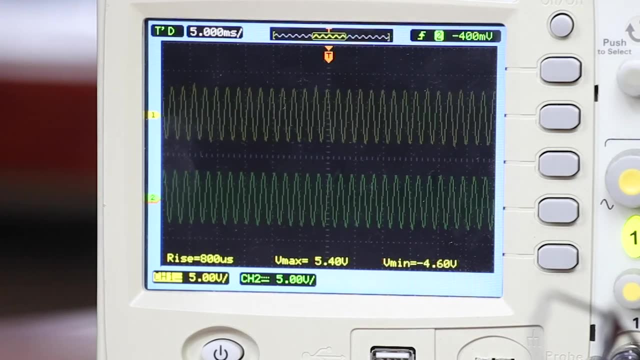 signals from two sources. I have amplifier one and amplifier two here, And at the moment they're both putting out 500 hertz, And that's why these two wave patterns are exactly the same, And so what we have here is the distance between them. here represents the period, And so therefore, if I 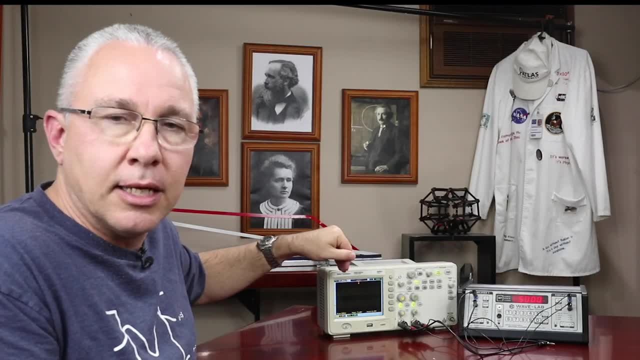 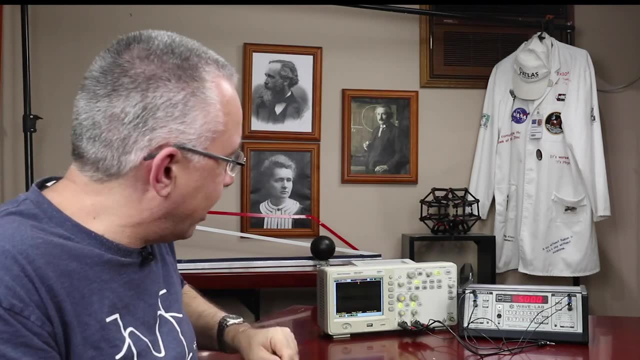 change the frequency, we're going to see a change in the pattern. So if, for example, if I have a lower frequency, that means also my period is going to be longer. I'm going to show that because on the top I have the left side and the bottom I have the right side, and I'm going to make the 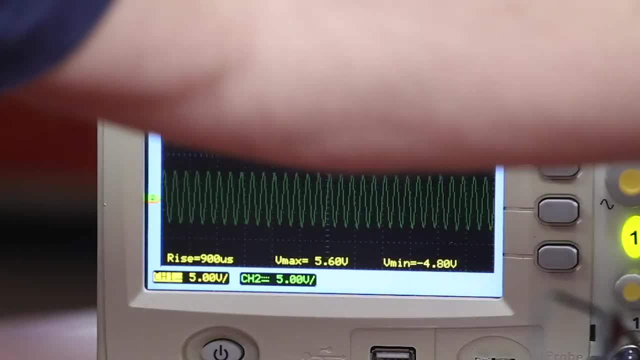 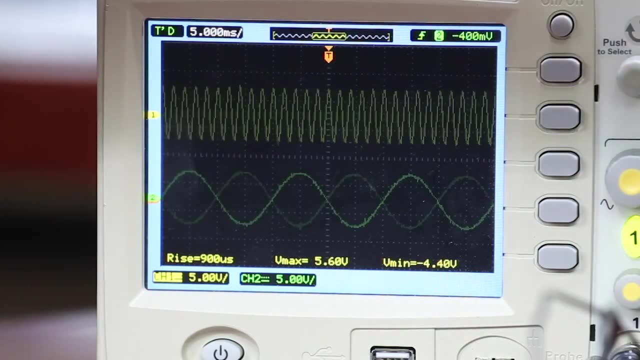 right side, not 500 hertz but 50 hertz. So straightaway you can see here that the period is longer, So the frequency is lower And of course it is 50 hertz If I were to measure the distances. 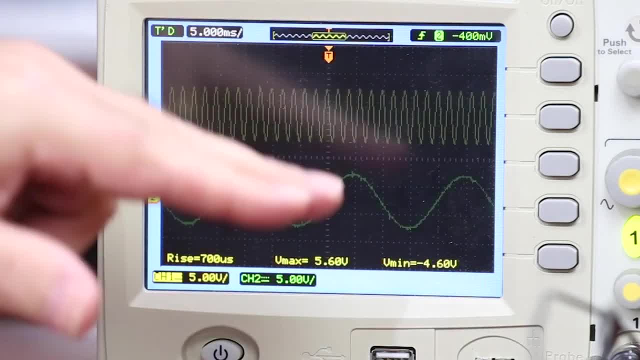 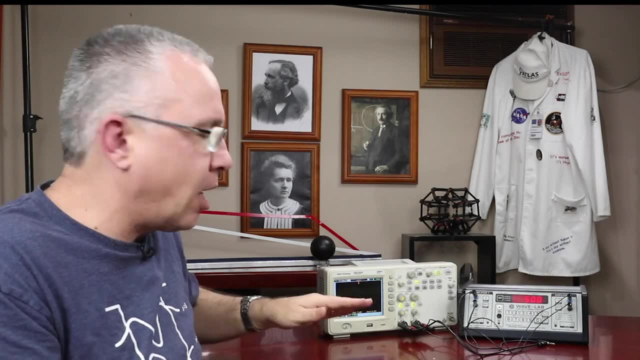 between the peaks. the distances here would be 10 times that one. Now, the first thing, what I do is I want to show you what modulation is not. So what I'm going to do is I'm going to add those two waves. That is what we refer to as superposition, And I can simply do. 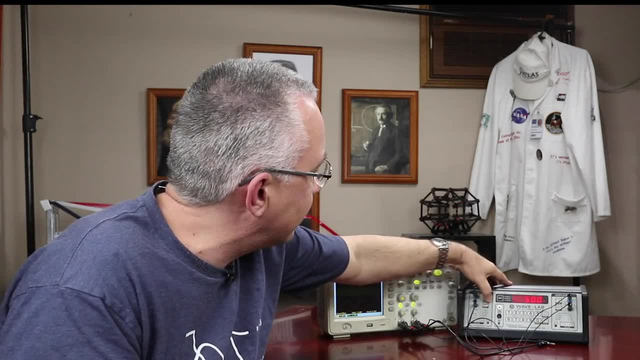 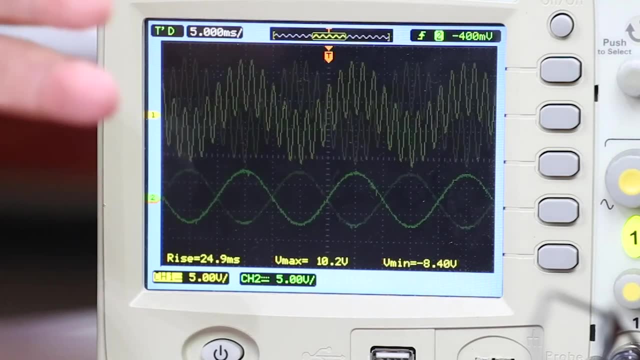 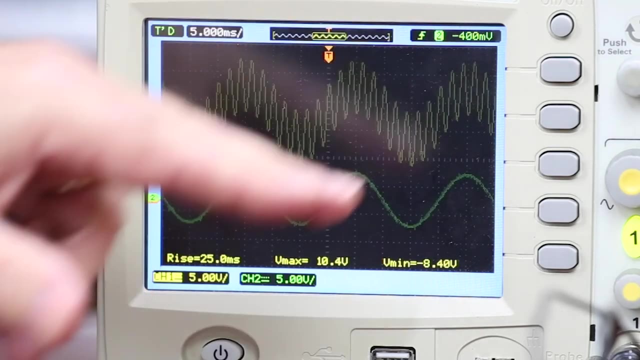 this by my box over here And I'm going to change that section to adding: And now what you see is we have the information down the bottom as a single, obviously single frequency tone and it seems to be superimposed on the top And you can see that the frequency of my carrier wave is still. 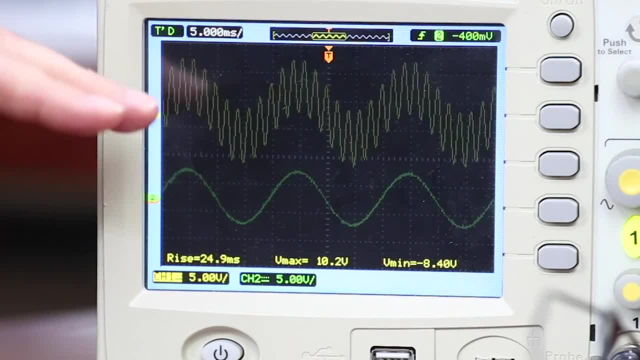 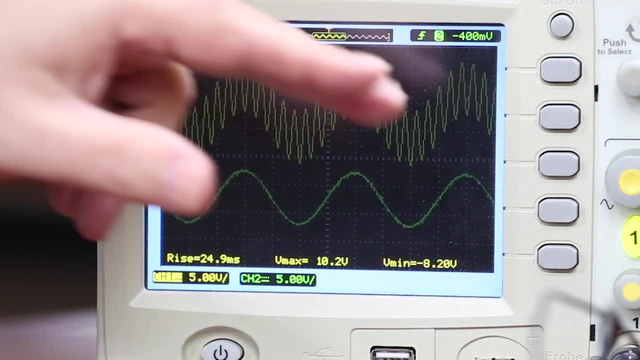 the same, but the whole frequency is the same. So I'm going to change that, And then I'm going to change that. So the whole thing is going up and down And, as a result, you can actually see two sets of waves in there. There's the, obviously the wave that we had initially, And then we also have 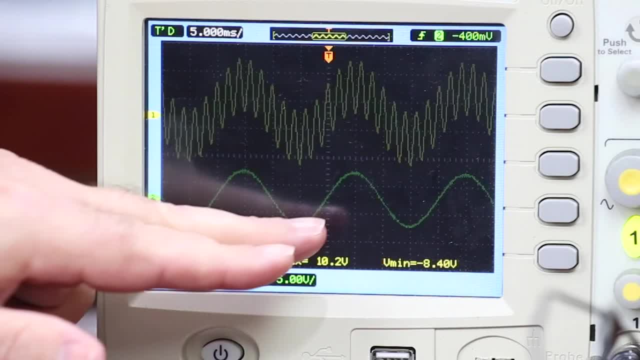 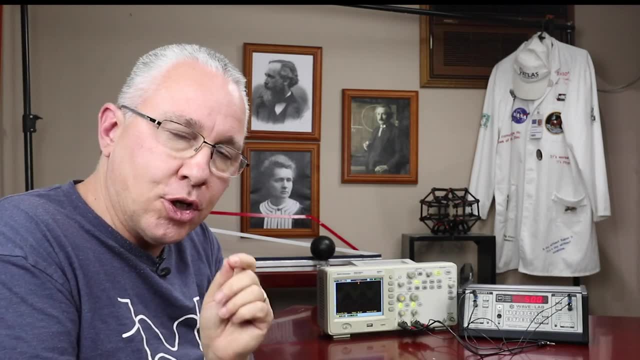 the fact that we have this period of these two peaks, which matches what we have here in the bottom. Now. that is not amplitude modulation. So what I want to do now is I want to show you what amplitude modulation actually looks like, So I can again change the settings here to do amplitude. 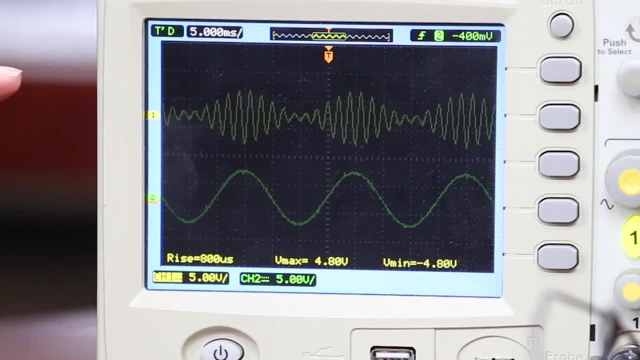 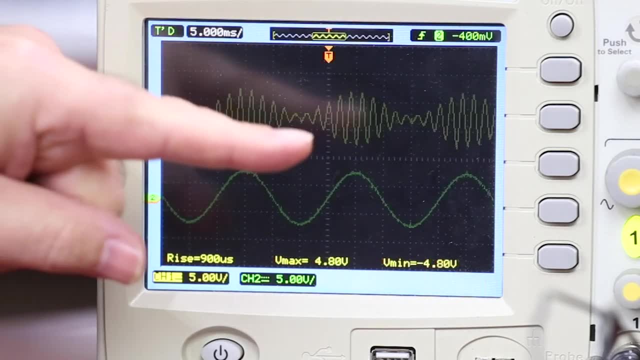 modulation. And now what you'll see is is that we still we don't have a wavy line in the sense of going up and down. We still have a wave, but the amplitude is changed. If you look carefully, here we have the. 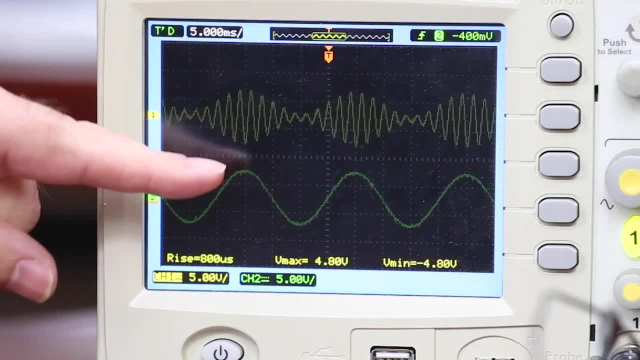 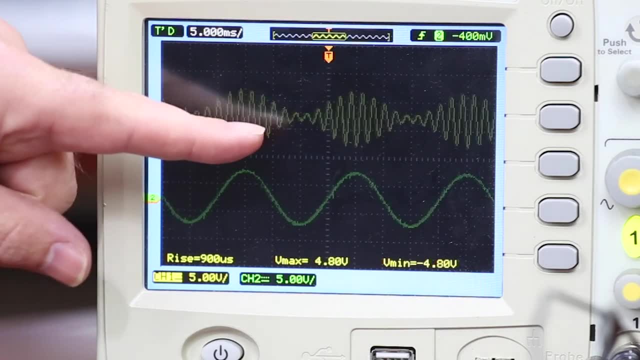 amplitude is a maximum and that corresponds to the peak of this signal. here, where we have a trough, or let's say, the bottom end of our wave, There we have a amplitude that is weaker. So what we have here is a changing of the amplitude that carries the information. 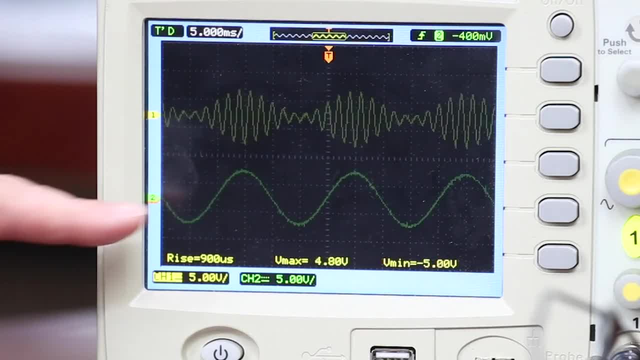 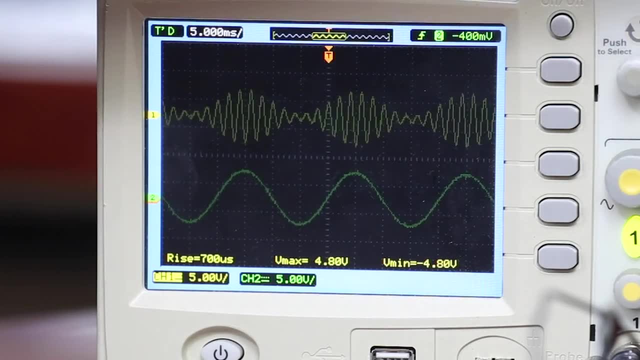 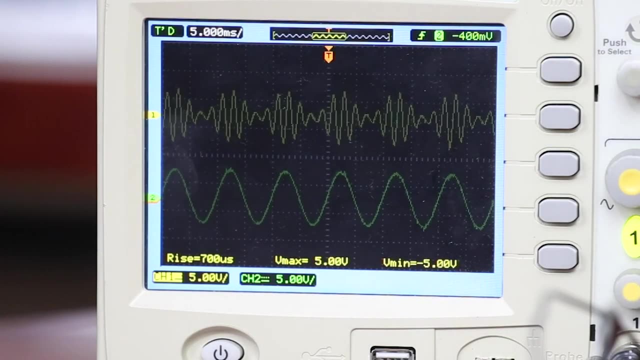 Of the signal down the bottom. If I were to change the frequency of the bottom wave- and we're going to do it- by simply multiplying this by two, So we're going to go to 100 hertz. You can see now that the period differences of the original signal is still the same. 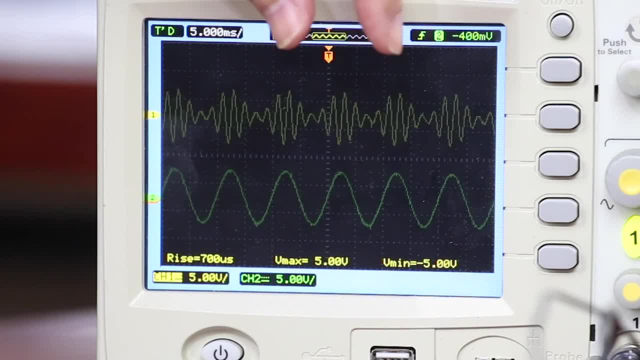 but the amplitudes actually now fluctuate at a greater rate And again it still matches the signal over here. So this is what we refer to as amplitude modulation. Now, this, I will say, is a very basic signal. It's a single frequency. So the sounds that you hear. 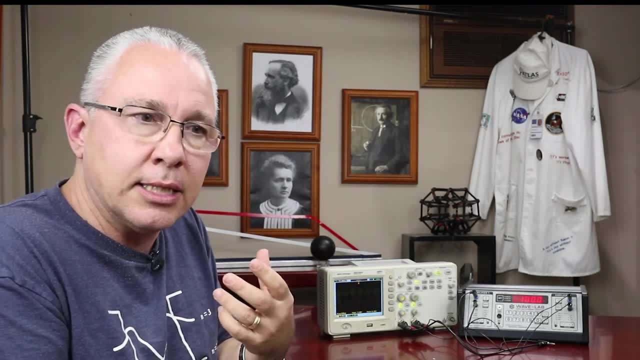 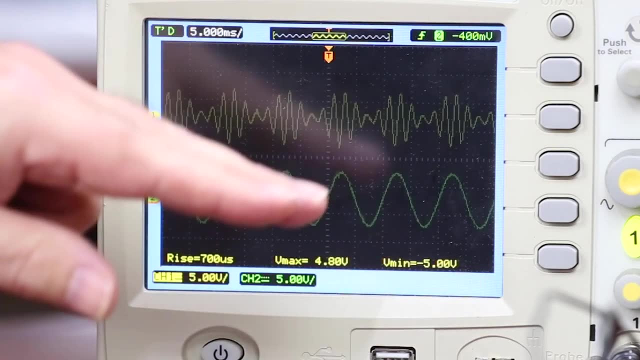 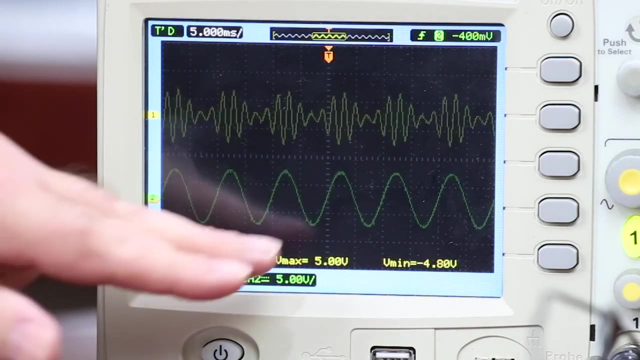 from the radio. the sounds of any sorts of more complex sources are going to be a much more complex wave pattern here, But nonetheless the wave pattern is such that the amplitudes in the carrier wave will match the patterns that are below it, Or in this case, what our signal is here. 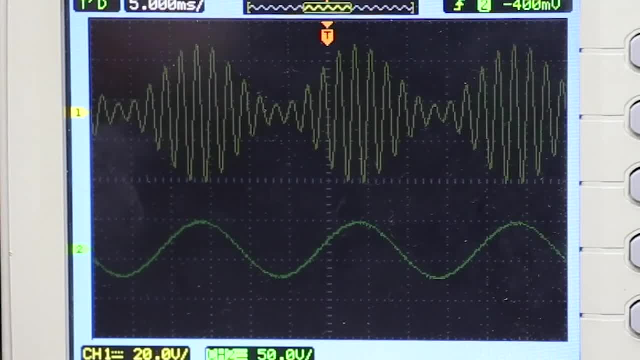 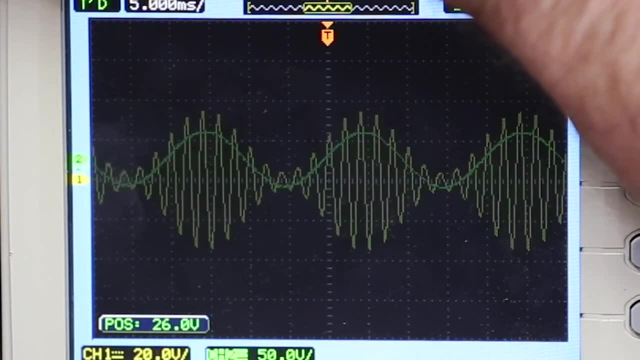 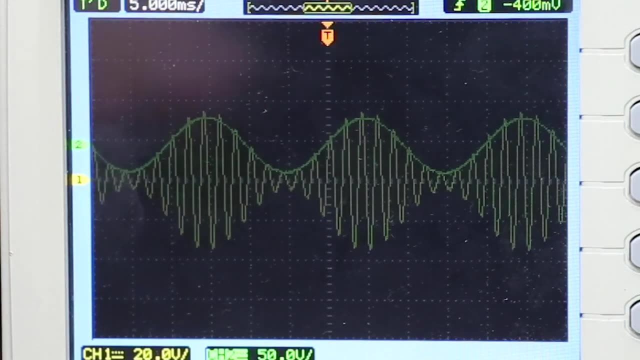 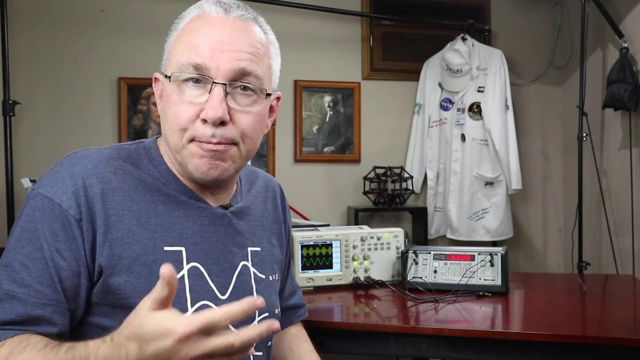 Let's overlay the two so that we can clearly see how the two are related. So you can clearly see that the carrier wave changes in amplitude and matches the original signal that we applied to it. Now, of course, our source wave has a period and a frequency in. 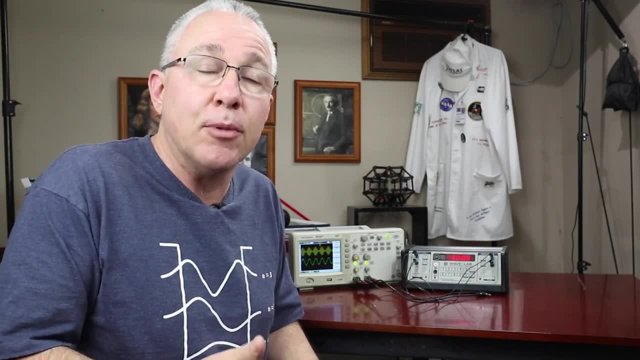 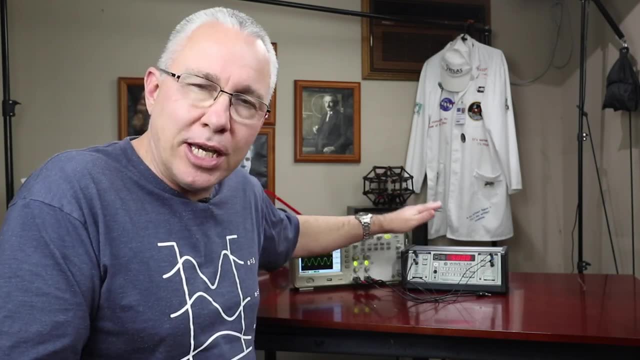 by association the wavelength, And of course we can determine that on the modulated wave. But of course our source wave also has an amplitude. Now there is a limitation here with this box, that if I change the amplitude of my source signal 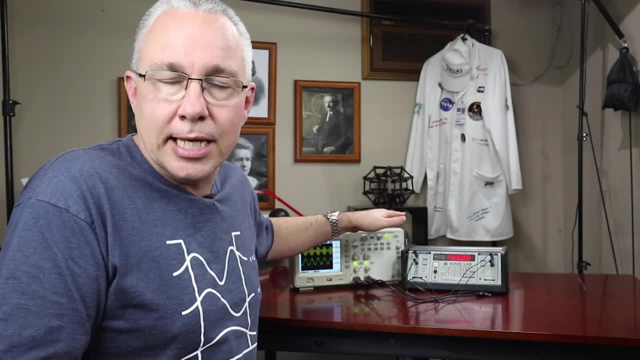 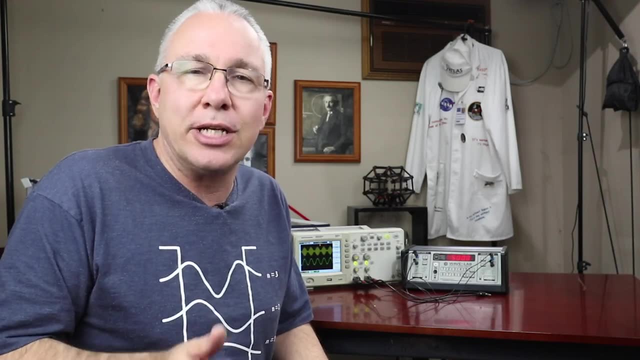 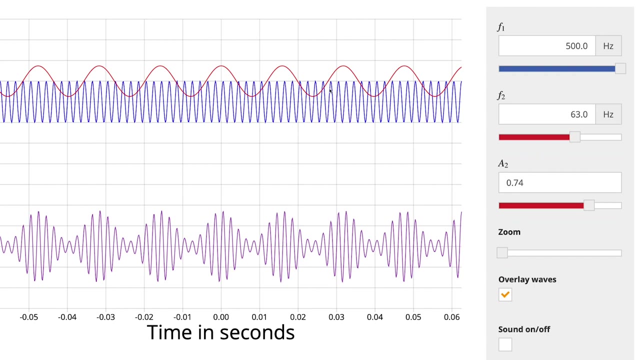 it won't accurately represent what the modulated signal does. So what I want to do is show you an animation that shows you also how changing our source signal amplitude changes the modulated wave. So here you see three waves in this particular animation. The red wave is, of course, our signal or source wave. 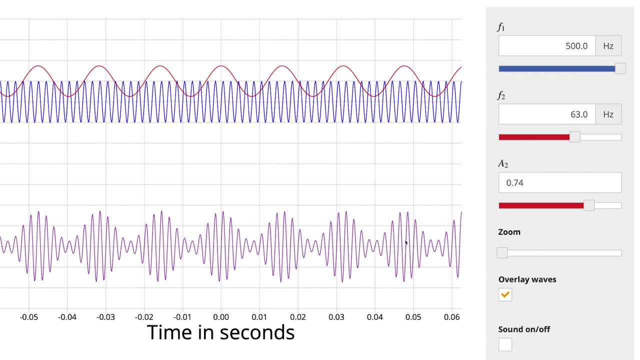 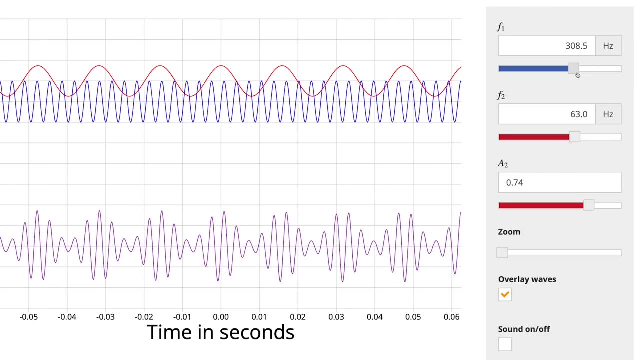 The blue one is our carrier wave And then we have our modulated wave down the bottom, going to change the frequency, in this case here, of my carrier wave, and you can see the modulated wave matches that. Similarly, if I change the frequency of 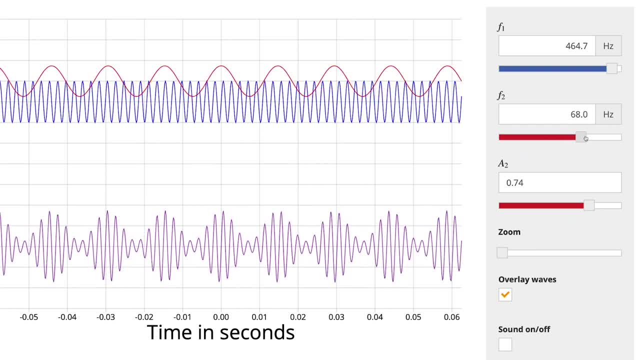 my signal or my source wave. you can see that also changes the modulated wave. The point I want to make here, though, is how amplitude of the source wave changes the modulated wave. Now, the first thing you'll notice is that if I change the 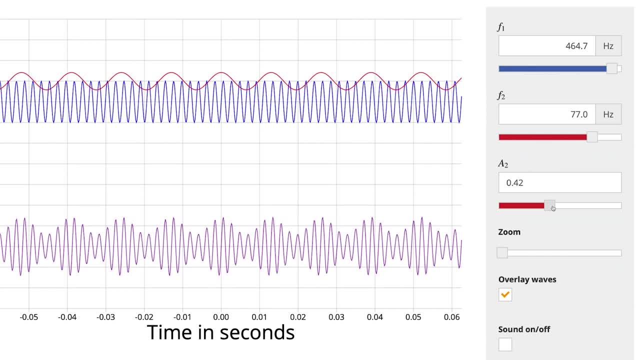 size of my amplitude, you will see that the maximum peak of my modulated wave gets larger and smaller. But the other thing you should notice is that the peak of the minimum also changes. So in low amplitudes the difference between the maximum and the minimum amplitudes is smaller. So if I have a larger 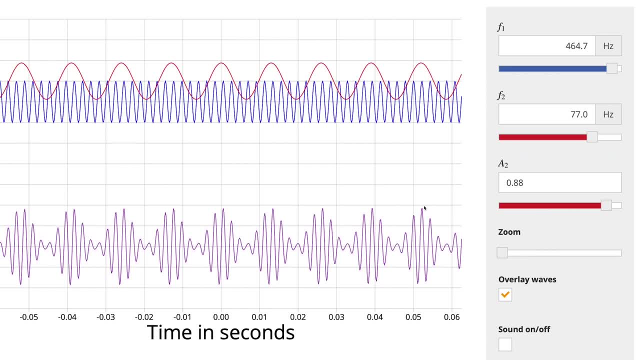 amplitude of my source signal. you can see the maximum amplitude is a lot bigger, but the minimum amplitude is smaller. So we have a greater difference between the minimum and the maximum amplitude as the amplitude of the original source wave increases. And so that's how the modulated wave encodes the amplitude of our source wave. So as 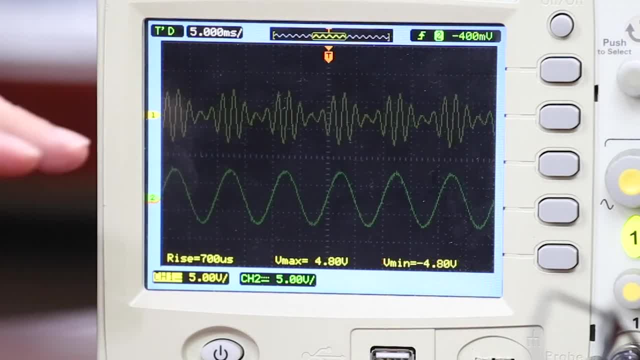 a quick summary. we have a signal here. a modulator takes that signal and uses it to change the amplitude of the carrier wave so that the changes in the amplitude match the pattern of the wave. And so, of course, at the other end, if you receive that signal, you can then have a demodulator which is able to extract. 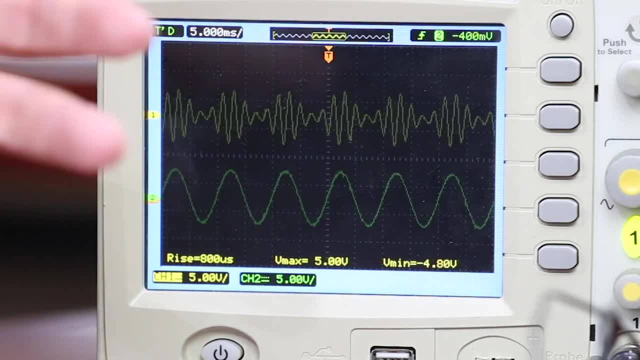 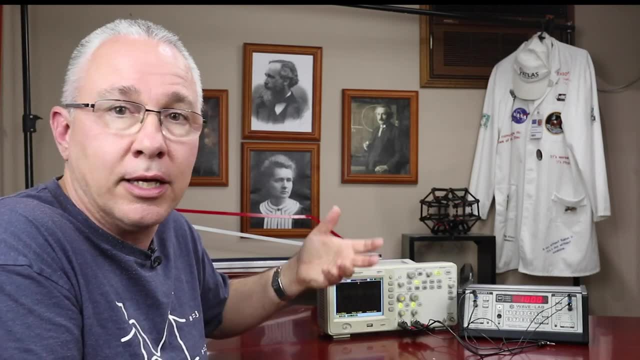 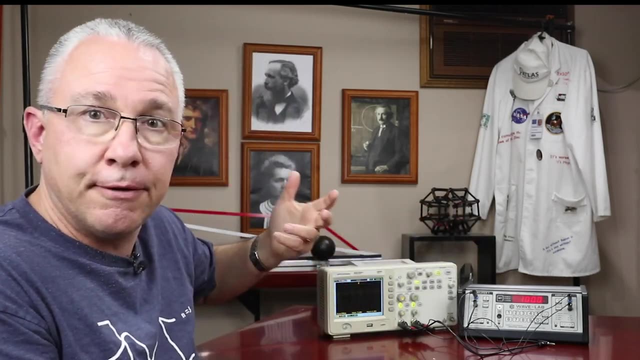 that information to give us back our original wave, And so therefore, it's an easy way of transmitting information, like our music with the light and of course also like in listening to your AM radio. But now let's examine frequency modulation. So again, I'm going to return this back to 50 Hertz and we have the 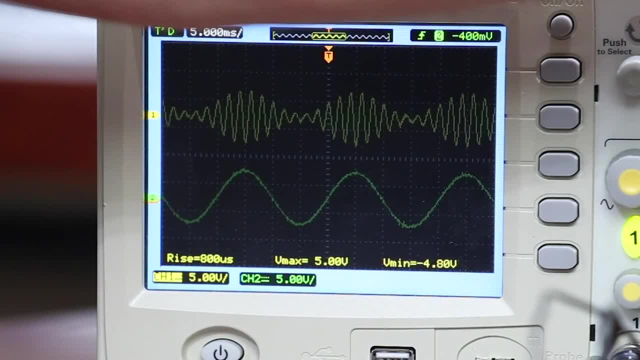 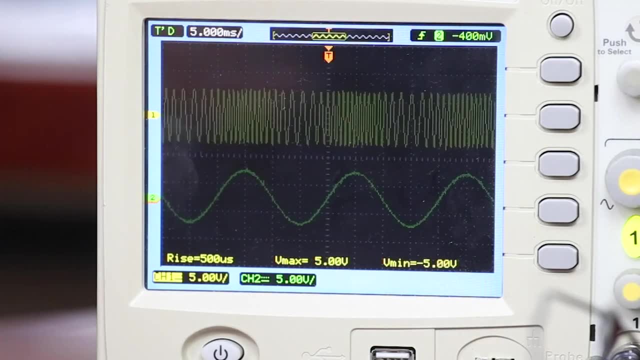 this pattern, But now I'm going to shift this to frequency modulation. Now, what you notice now is that the amplitude of my carrier wave does not fluctuate at all. it stays constant. But if you look very carefully, is that the pattern of 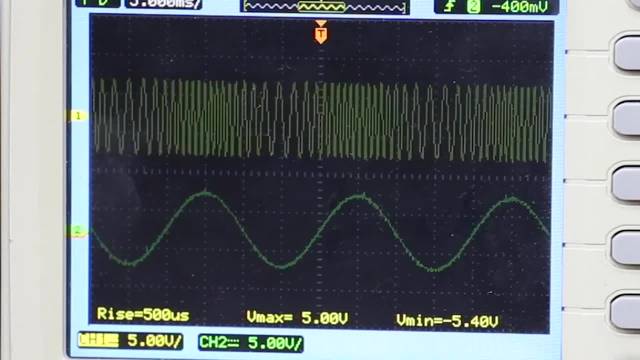 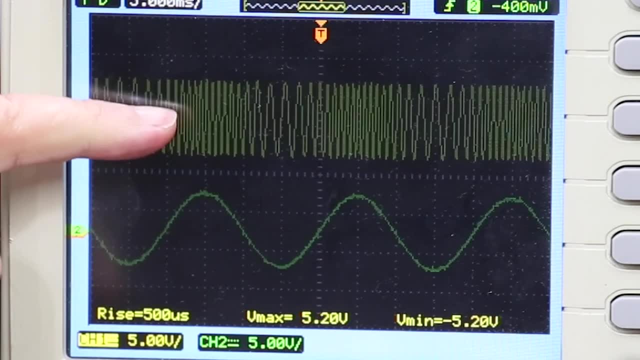 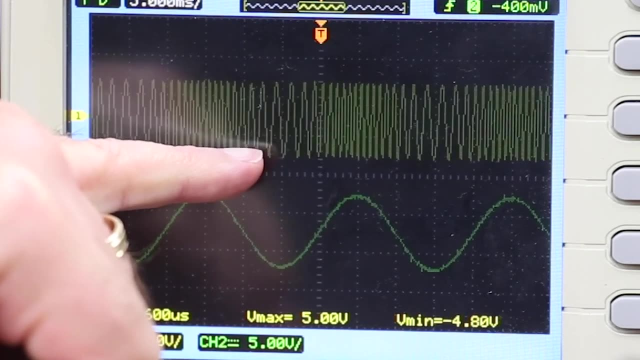 frequencies or the periods we could talk about as well, changes in respect to the wave down the bottom. So if you look here, at the peak here is that the frequency is actually a little higher there, Whereas at the bottom of this section, here, you'll find that the frequency is a little lower, so you can see a repetitive 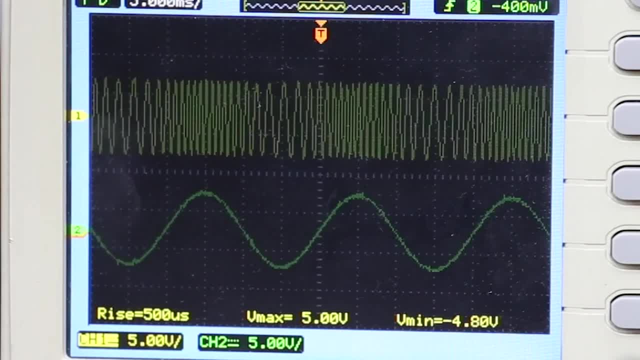 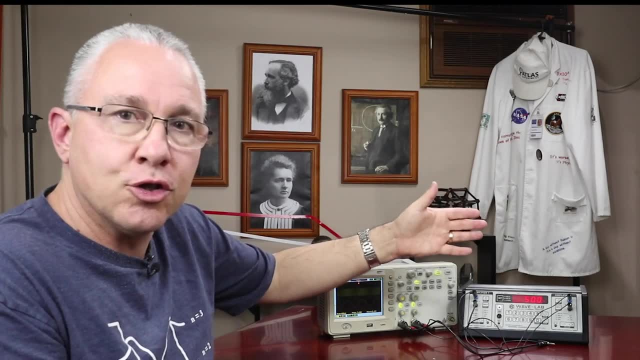 pattern that matches the pattern down the bottom. And what is happening is the frequency is changed, the frequency is modulated. And so if I now change the frequency of my source signal- let's say 100 Hertz- let's see what happens to our 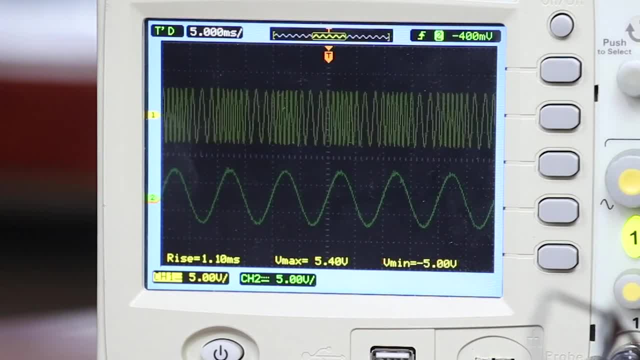 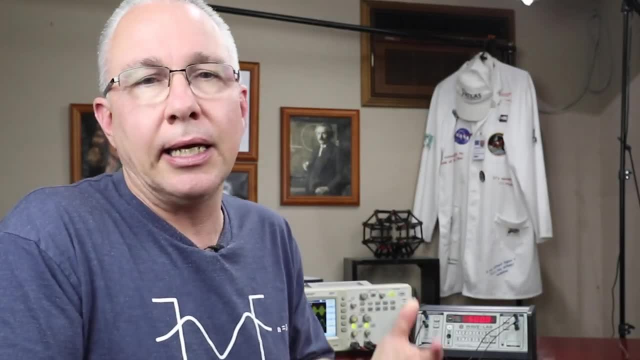 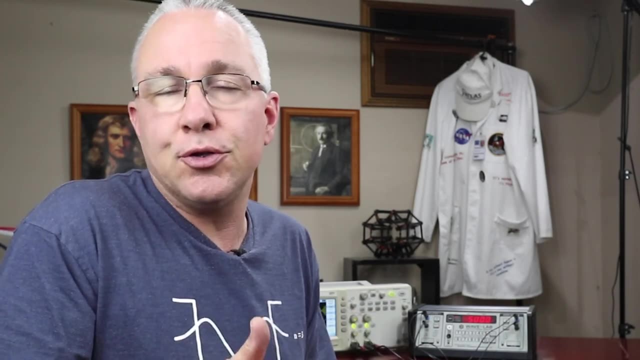 frequency pattern. So now you can see more clearly that the pattern is matching the bottom pattern. Now, similarly, in terms of frequency modulation, the amplitude is also encoded in the waveform, so you can get both the amplitude and the period, which therefore by association allows us also to work.